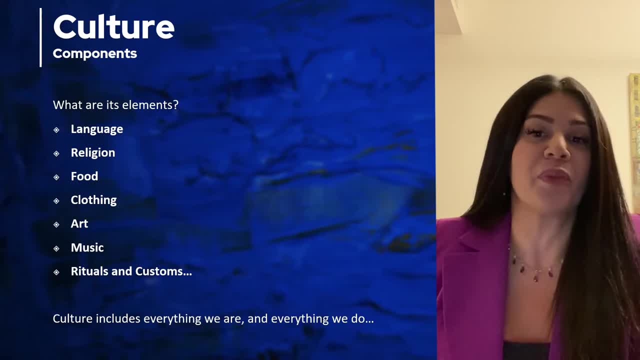 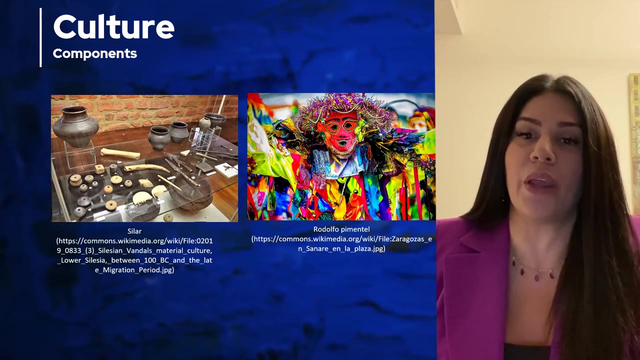 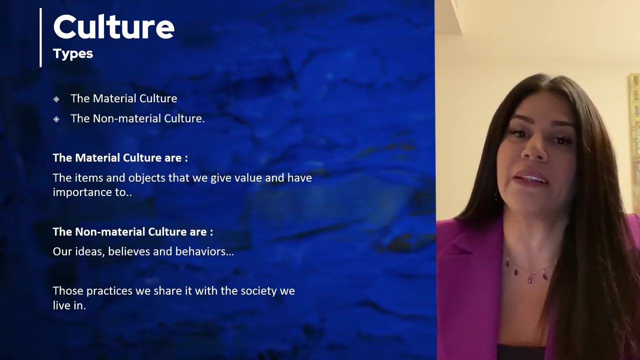 So culture includes what we eat, how we dress, what we speak, where we live, how we interact with our family, how we organize ourselves in the group, and so much more. Culture includes everything we are and everything we do. In the essence of the term, each object in our body is something external. 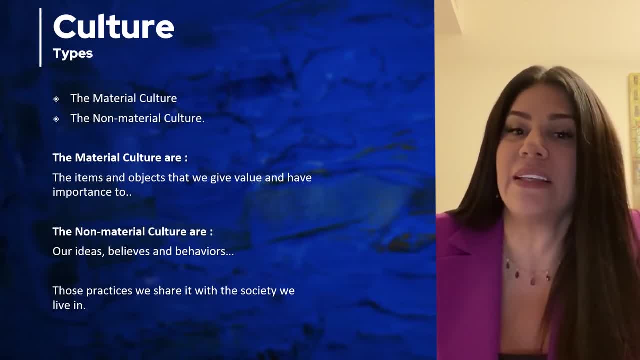 To be clear in culture, or盧 is an overlay of theти arte professor In movie theater and the movie yokai, in这说法 meaning to all, superdel enjo. Since, let's put this straight to the fabric of culture, culture could be divided into two main categories: the material culture and the none material culture: The material: 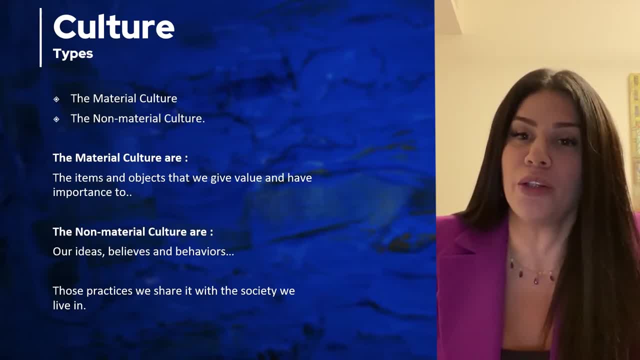 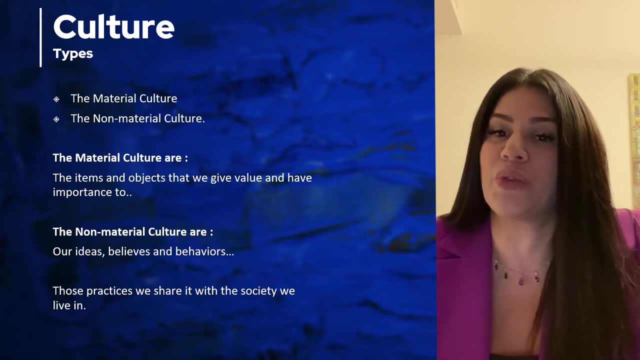 culture are the items and objects that we give value and have importance to, things that we're wearing and that we're using, things that we purchase it and we see it like more important than other objects, While non-material culture, on the other hand, focuses on our ideas and our belief. for example, how do you celebrate? 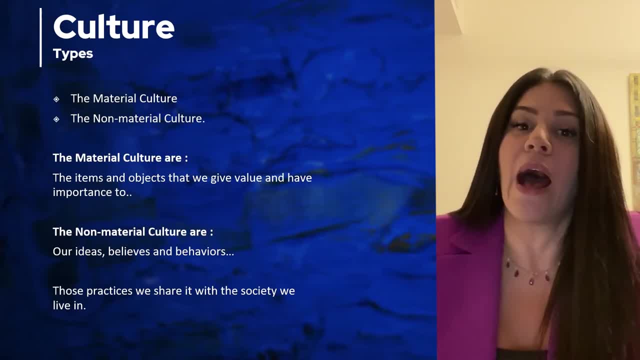 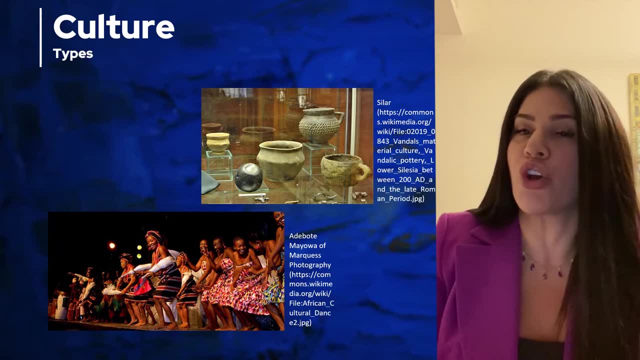 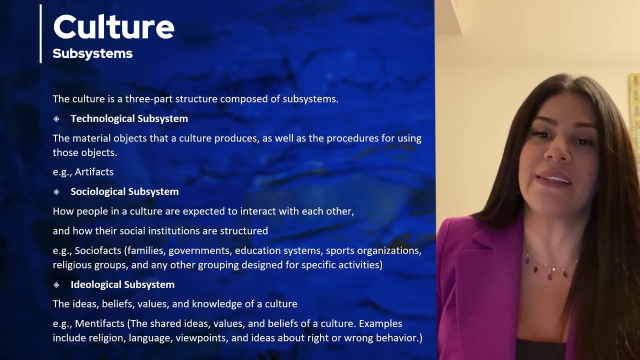 holidays or big life events? how do you celebrate weddings? what you do when someone is having a new baby or getting a new job or getting married. these are non-material culture, those practices we share it with the society we live in. the anthropologist leslie white suggested that a 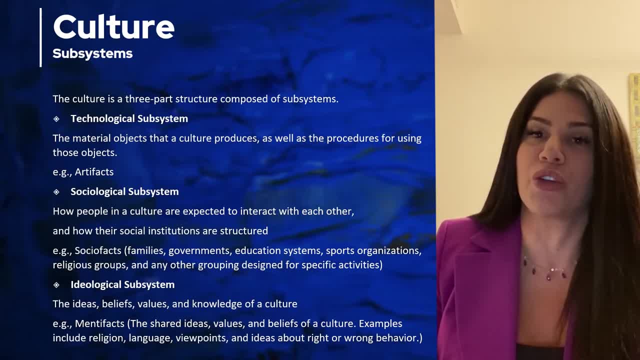 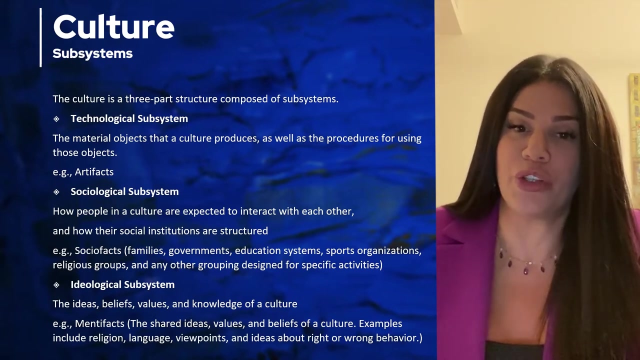 culture could be viewed as three-part structure composed of subsystems. we have the technological subsystem, sociological subsystem and ideological subsystem. technological subsystem: the material objects that our culture produces, as well as as as as as the procedures for using those objects. we call them artefacts. 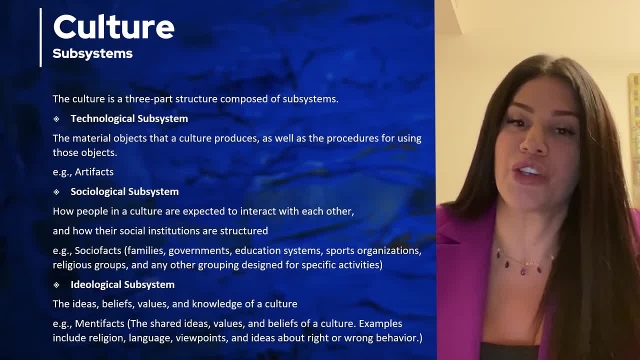 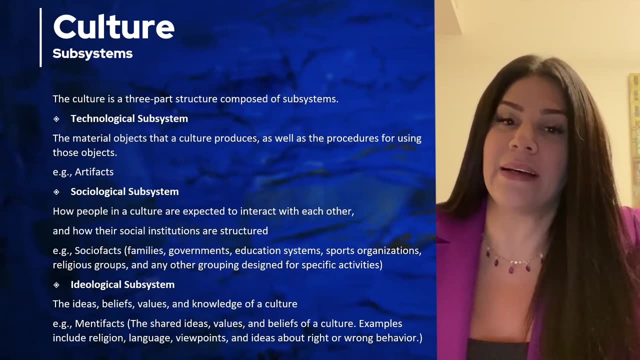 Sociological subsystem: how people in a culture are expected to interact with each other and how their social institutions are structured. we call them socio-facts. Ideological subsystem: the ideas, beliefs, values and knowledge of a culture. we call them mentee facts. 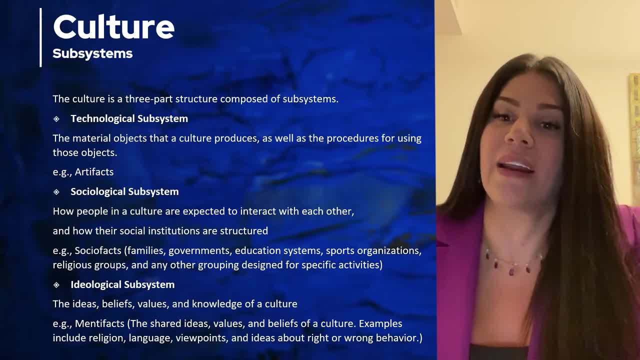 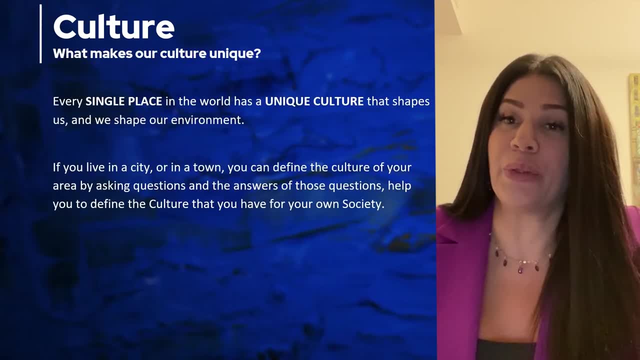 Those are the system of culture. they are integrated and each reacts on the other. Every single place in the world has a unique culture that shapes us and we shape our environment. If you live in a city or in a town, you can define the culture of your area by asking: 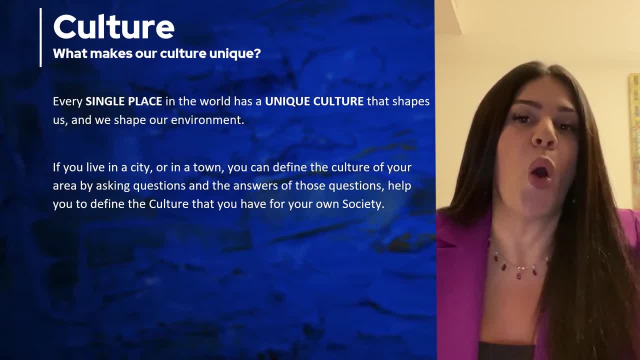 does your city have public transportation? What type of buildings are available? What type of homes do people have? What is the type of agriculture there? It is a modern city. Do you have a busy downtown? Are you in an urban location or in a rural location? 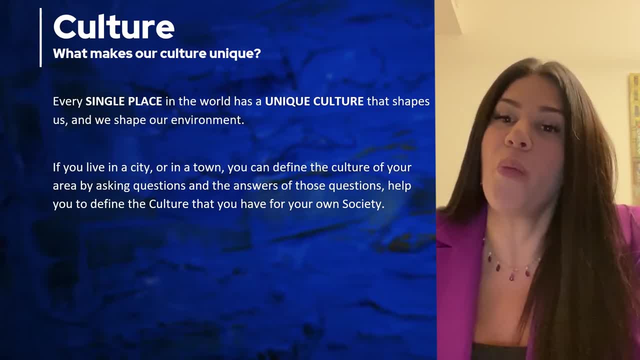 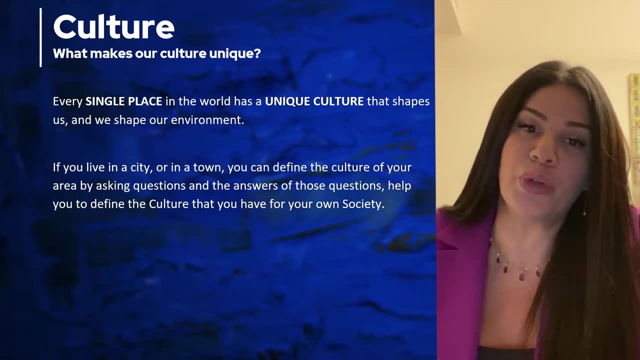 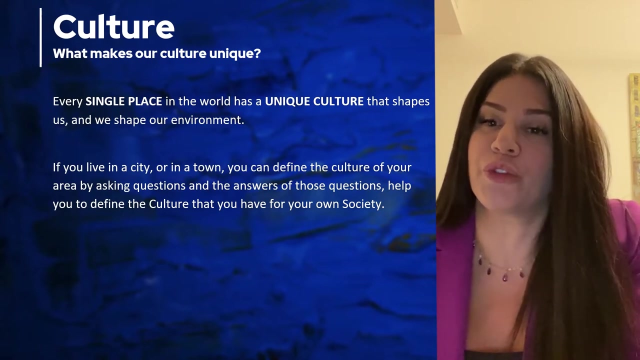 How is the land used in your city? How do people in your society interact? Are people interacting more through technology? What language is spoken in person? What clothes are in style? What music is popular? What religions are prominent in your society? What food people eat? 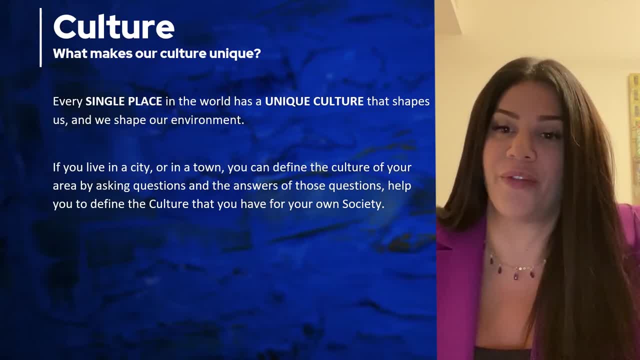 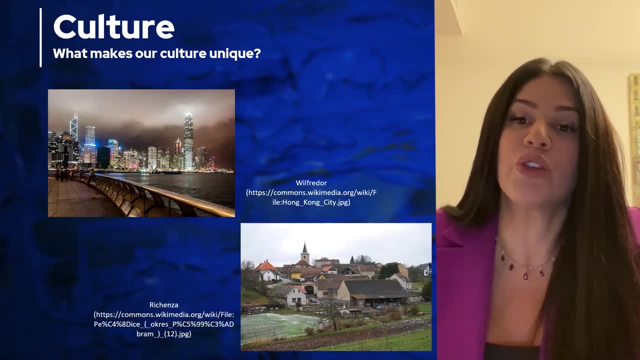 What type of government do you have? What is allowed in your society and what is not allowed? What type of money is used? What social norms does your society have? does your society have, and what jobs are offered in your society? the answer of those questions. 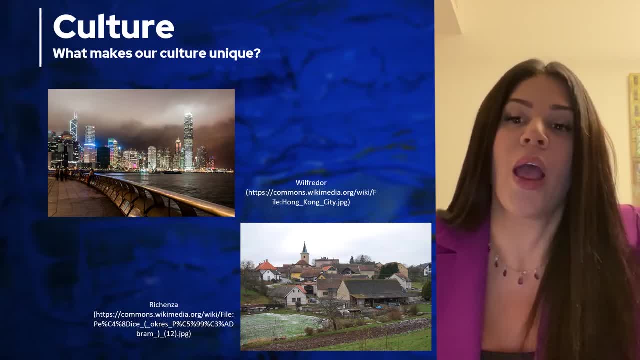 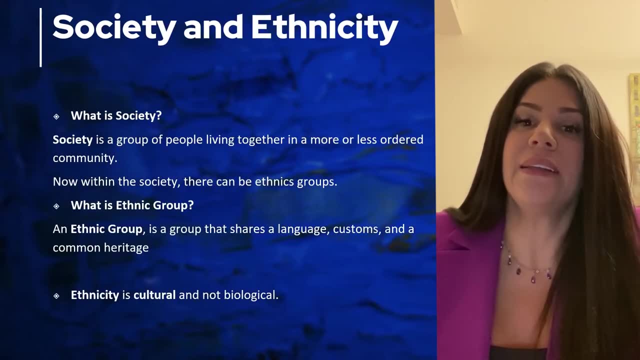 help you to define the culture that you have for your own society. What is society? Society is a group of people living together in a more or less ordered community. So when we talk about the society, we're talking about the group of people that organize themselves through laws or several. 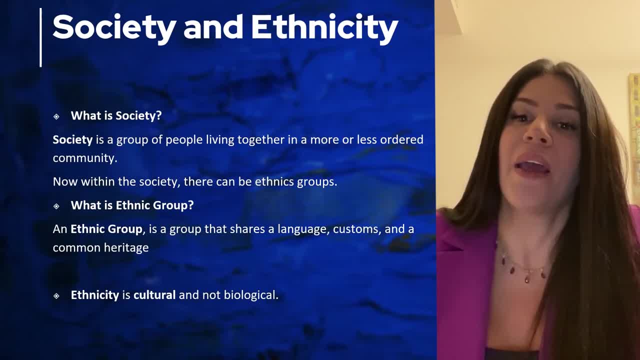 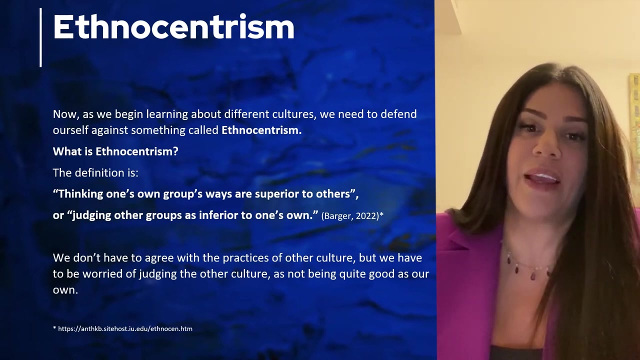 rules. Now, within the society there can be ethnics group. An ethnic group is a group that shares a language, customs and a common heritage. What interesting is that ethnicity is cultural and not biological, Dr Evelyn Heyer said. Now, as we begin learning about different cultures, we need to defend ourselves against something. 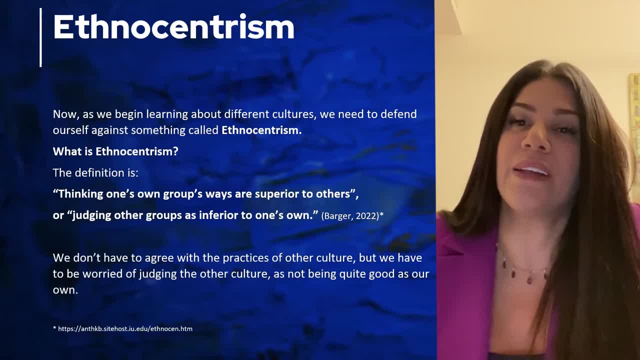 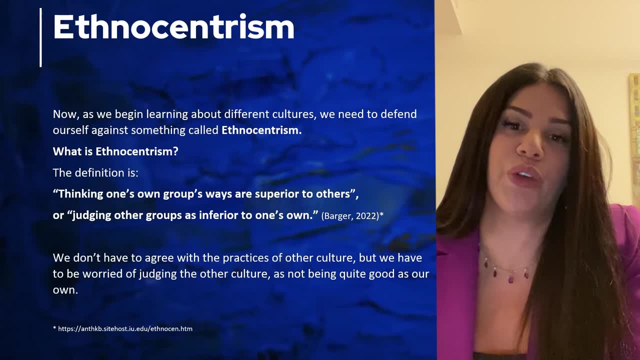 called ethnocentrism. Ethnocentrism is the idea that our own group or culture is better or more important than others. The usual definition of ethnocentrism is that it is a group of people living together in a more or less ordered community. The definition of the term is thinking one's own. 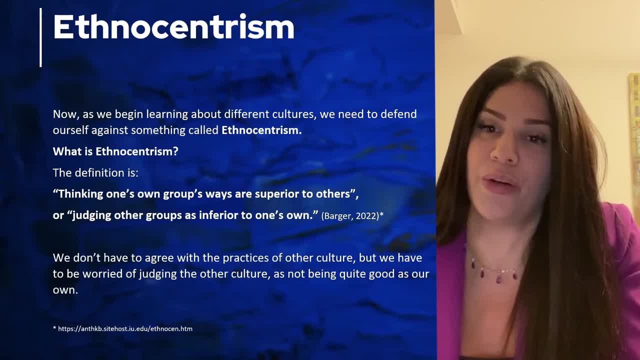 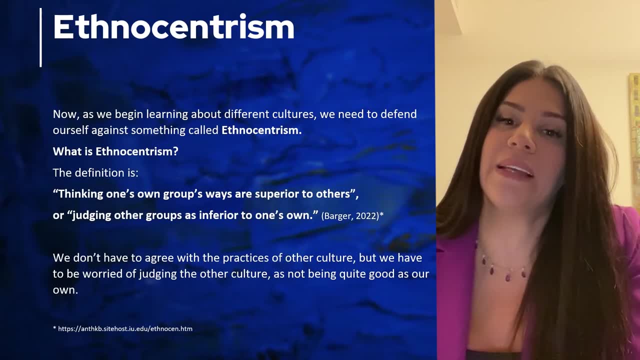 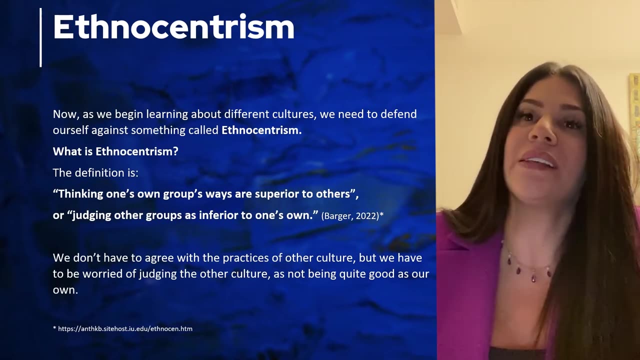 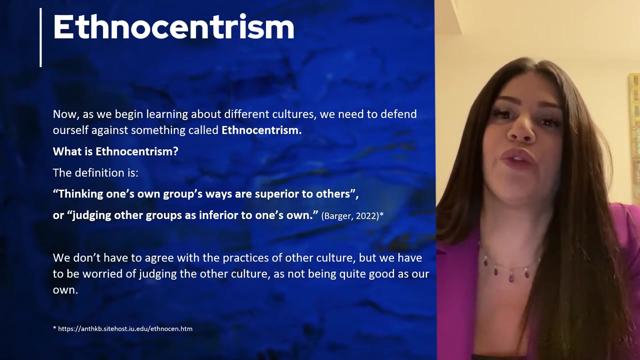 group's ways are superior to others, or judging other groups as inferior to one's own. The problem is, it's so easy to be ethnocentric. Let me give you a simple example. For example, the traditional Korean culture believes that red ink is only used for writing the names of people who are 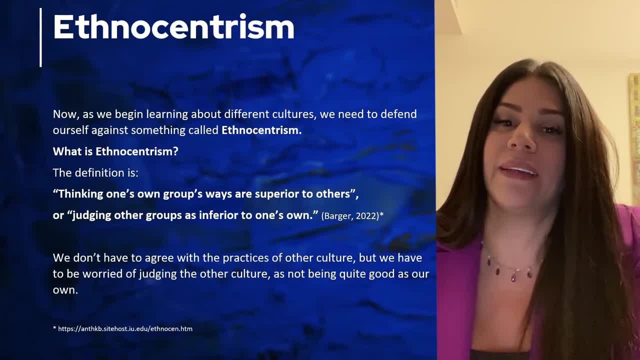 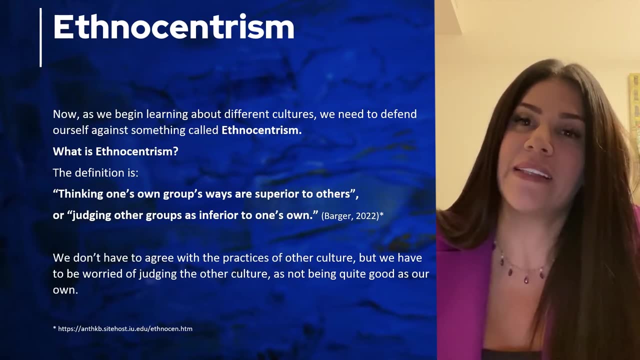 dead. Writing a living person's name in red is seen as wishing harm to come to that person. So it's pretty easy to think that maybe our own culture is better. That is ethnocentrism. We don't have to agree with the practices of other culture, but we have to be worried of judging the other. 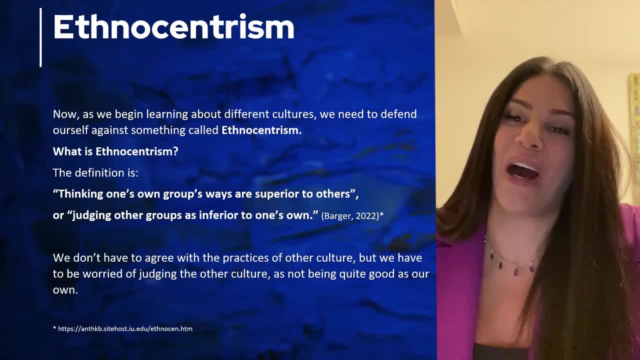 culture as not being quite right. So let me give you a simple example. For example, if you have a large country where you are living with an ethical family, then you can be very specific with that Garden. For example, if you have a huge Chinese immigrant family and the name of the person 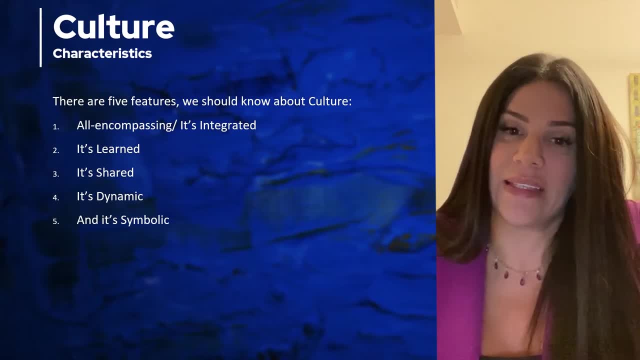 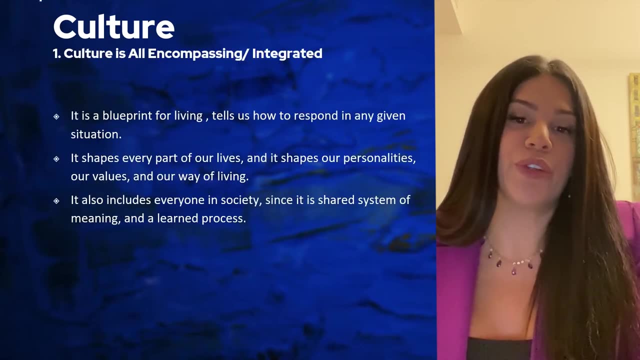 you are living with is Ethan. you can put Ethan in there and they think that they are not the most sociable. And you can put Peter here and they can say that they are the least sociable. If you just put Peter in the middle, you can say that they are not the most sociable. 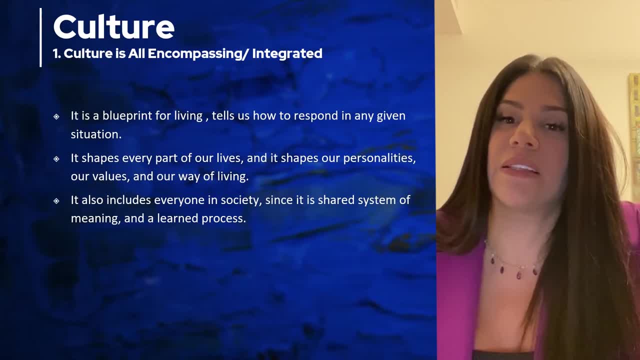 And when you put Peter there, you can also put Ethan in there, And when you put Peter in the middle, you can put Ethan there- Either that person or you can write that person down. And so it's very easy to think that encompassing this means that it shapes every part of our lives and it shapes our personalities. 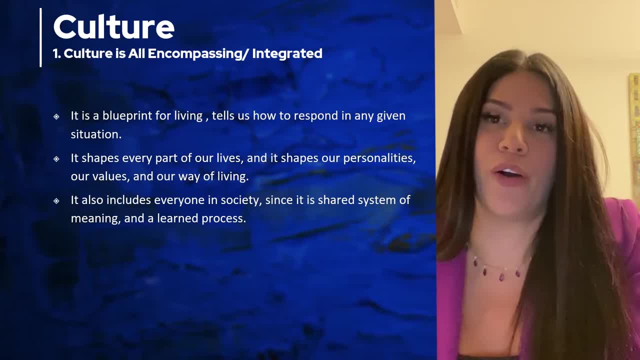 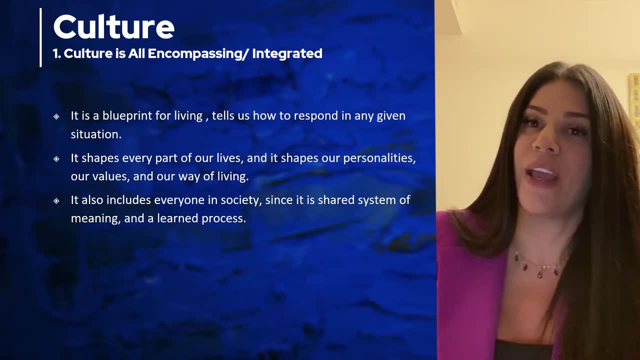 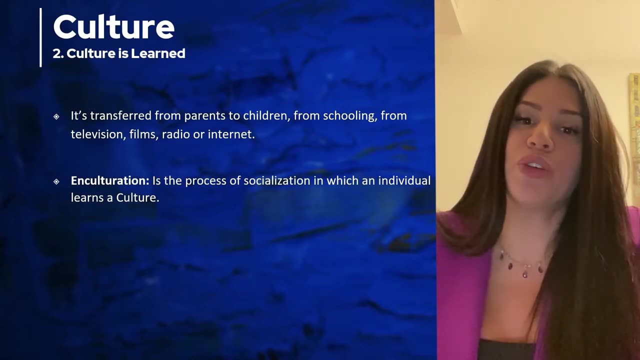 our values and our way of living. this means that it also includes everyone in society, since it is shared system of meaning and a learned process. culture is learned. we should also understand that culture is learned. it's transferred from parents to children, from schooling, from television films, radio, internet. we begin learning our culture from the moment. 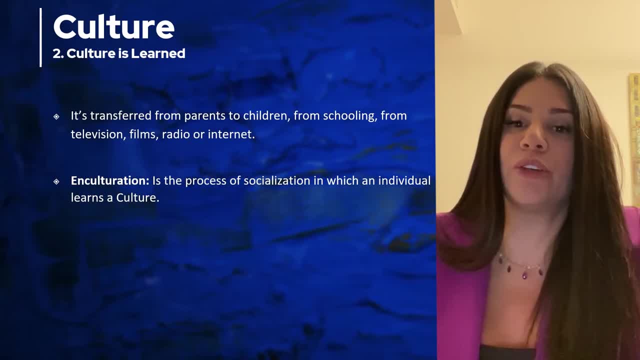 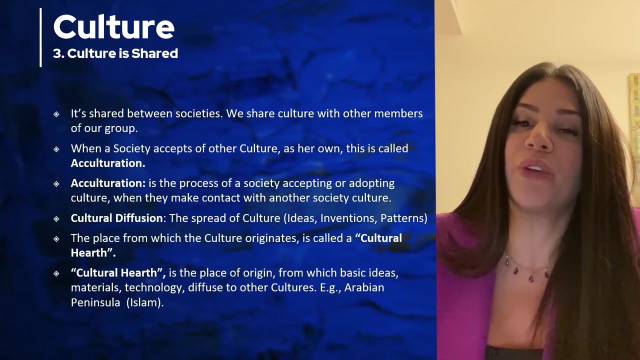 we are born as the people who raise us, encourage certain behaviors and teach their version of right and wrong. this process is called inculturation. inculturation is the process of socialization, in which an individual learns a culture. culture is shared. it's shared between societies. we share culture with other members of our group. we are able to act in socially. 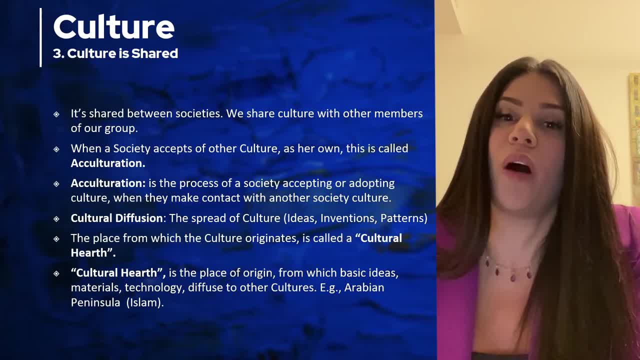 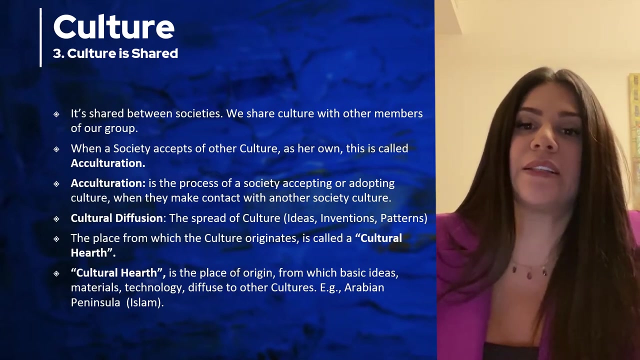 appropriate ways, as well as predict how others will act. despite the shirt, the shirt nation of culture. that doesn't mean that the culture is homogeneous. when a society accepts of other culture as her own, this is called acculturation. so acculturation is the process of a society accepting or adopting culture when they make. 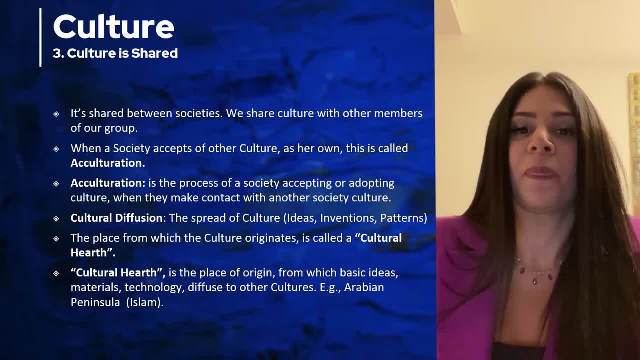 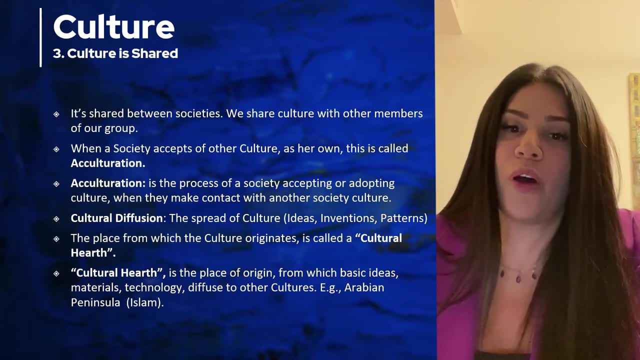 contact with another society, culture. this spreading of ideas, inventions, pattern is called diffusion, part of movement. if you remember, a movement team in geography and the place from which the culture originates and moves from is called a cultural hearth. cultural hearth is the site candy ever cabbage. 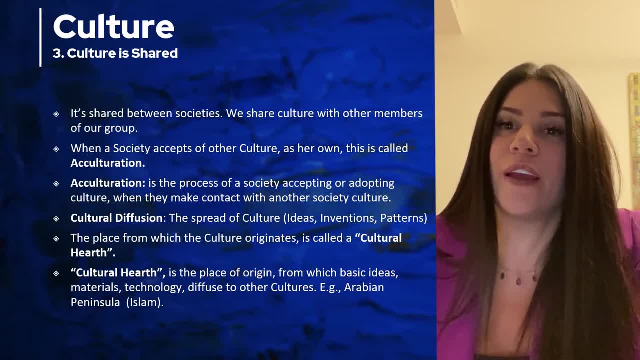 or of in Devimar, innovation, or the place of origin. from which basic ideas, materials, technology do you use to alter theа cultures? for example, Islam has a herd on the Arabian peninsula. that's why culture 줘 culture over the trainings. aBut when we think of devrait. 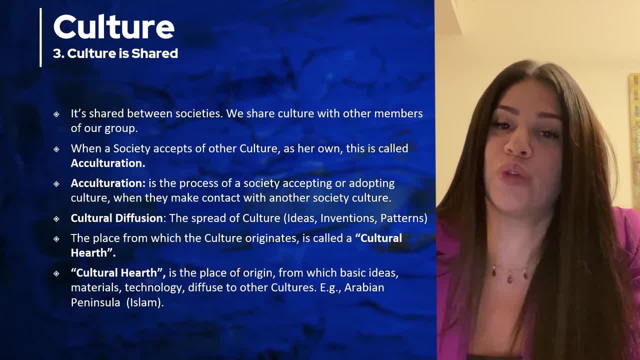 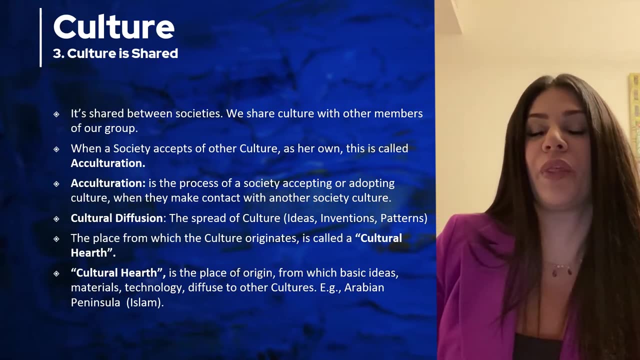 da mecca and medina are so important to islam, or in islam, it then spread to northern africa and south west asia. judaism and christianity are both from the middle east. their culture, heard, is the middle east. there are many different ancient cultural earth like mesopotamia in the middle east ancient 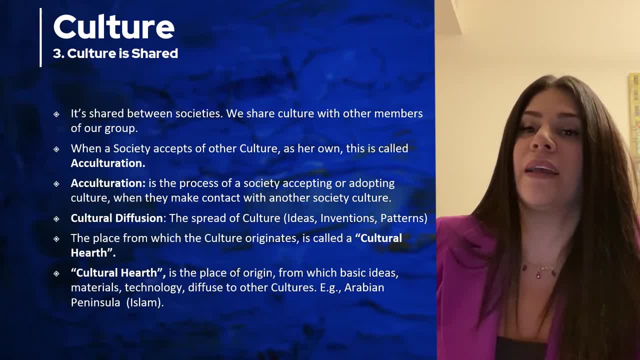 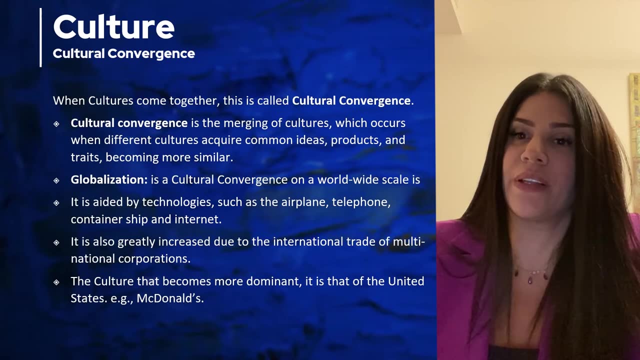 egypt in northeast africa, the indus valley, civilization of pakistan and india and the yellow river in china, etc. now, when societies have contact, which with each others and cultures come together, this is called cultural conversions. so cultural convergence is the merging of cultures with which occurs when different cultures acquire common ideas, products and traits, becoming more similar. 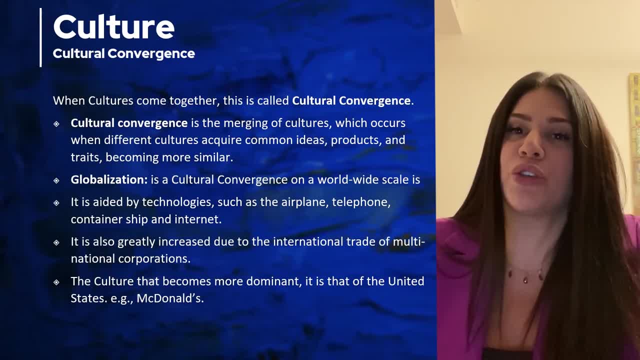 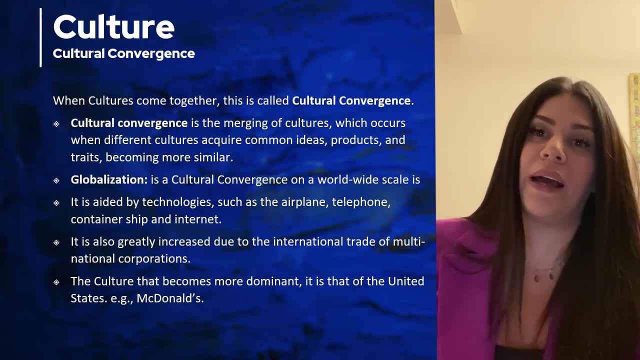 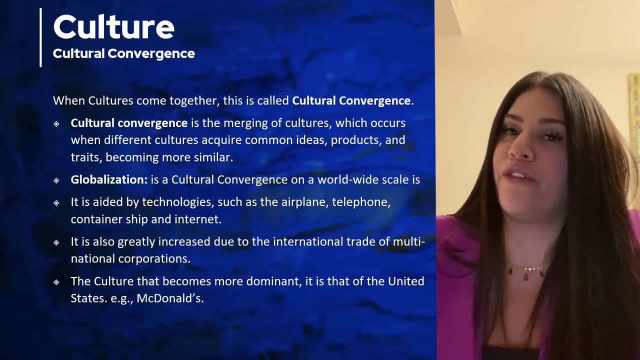 so cultural conversions causes cultures to become more similar, and cultural conversions on a worldwide scale is globalization. it is aided by technologies such as the airplane, telephone, container ship and internet. it's also greatly increased due to the international trade of multinational corporations. essentially, globalization is a cultural convergence. 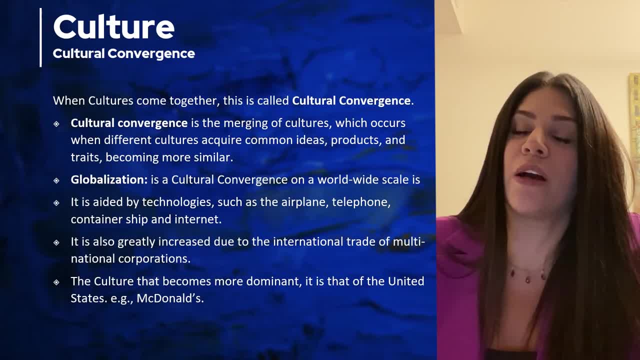 on a worldwide scale and the culture that becomes more dominant it's, it is that of the united states. uh, let's say uh, for example, mcdonald's thirds through globalization. mcdonald's went from being a local fast food restaurant in the US to global sensation in the fast food industry. 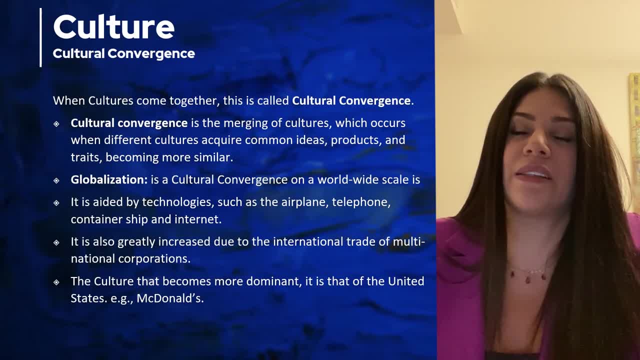 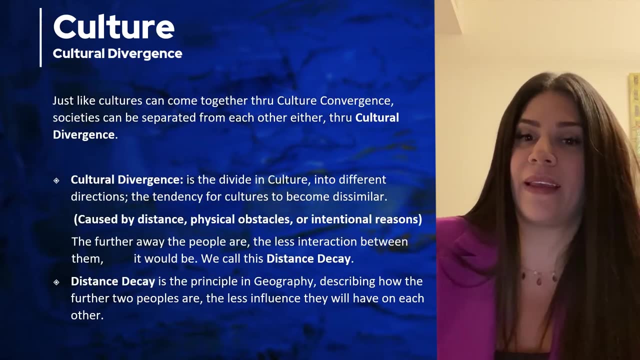 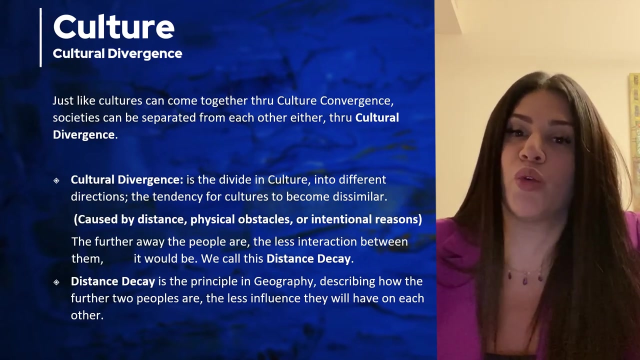 There are now McDonald's restaurants in almost every country. We can eat McDonald's in 118 countries in the world today. And just like cultures can come together through culture conversions, societies can be separated from each other either through distance, physical geography or from their own choice. 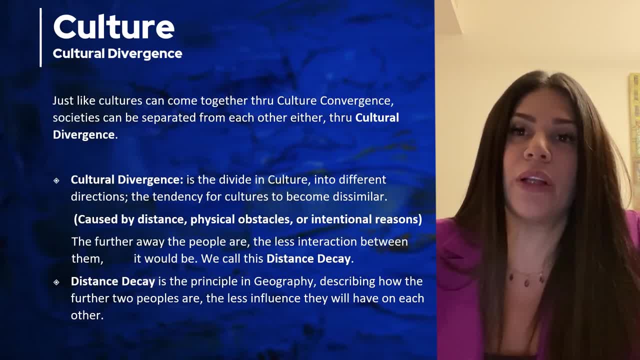 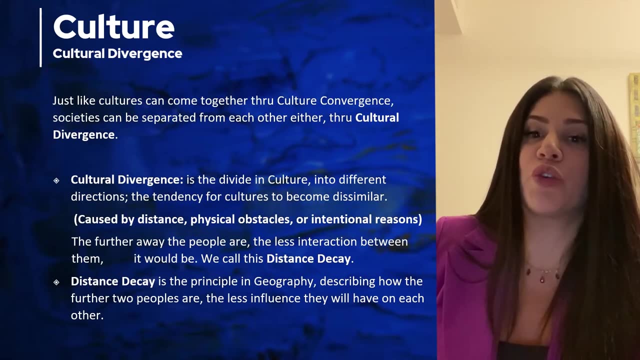 When this happens, we call this cultural divergence. So cultural divergence is the divide in culture into different directions, The tendency of cultures to become dissimilar, Education that focuses only on their own culture, rejecting other cultures, is an example of cultural divergence. 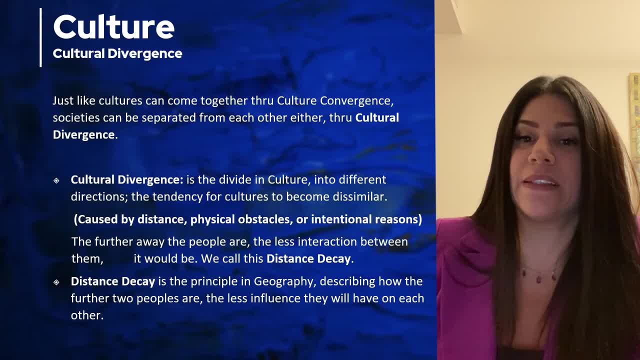 An example of cultural distance through distance or physical geography is when we have, for example, two places separated with a range of mountain. let's say, This distance between those two regions is called distance, This distance between those two regions is called distance. 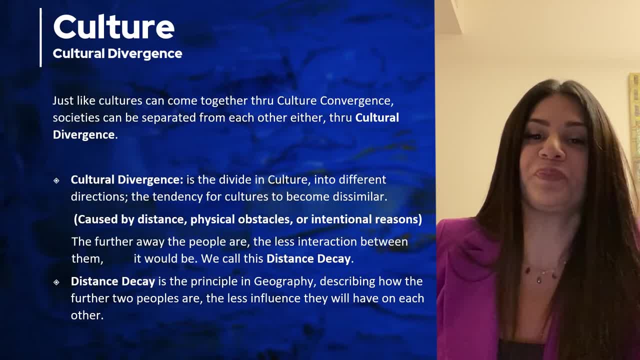 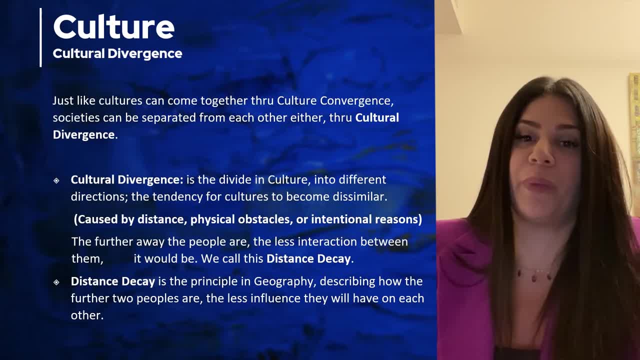 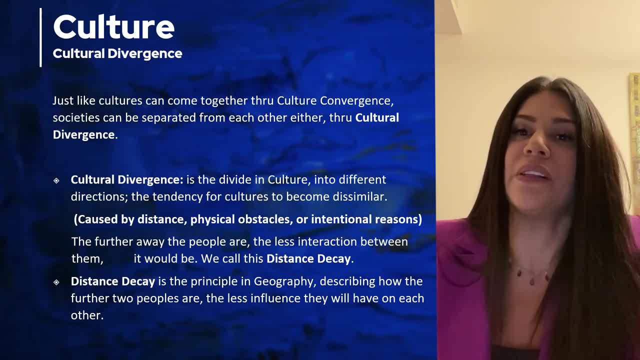 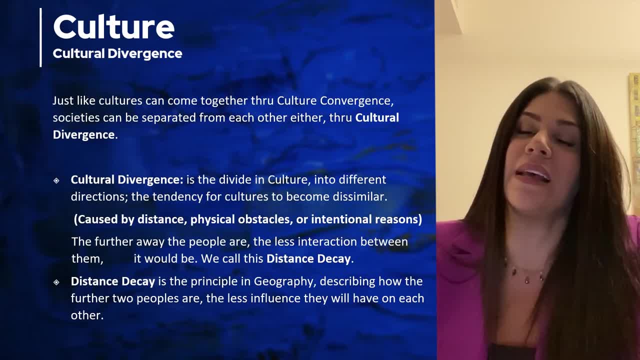 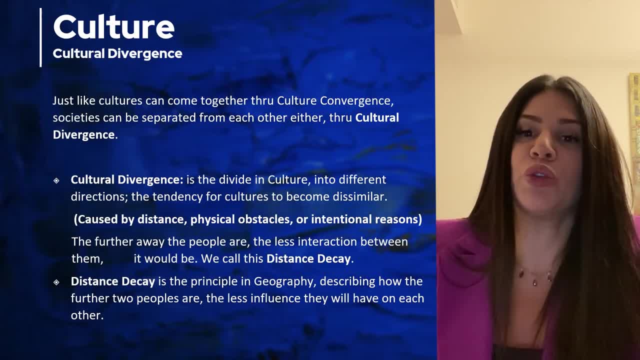 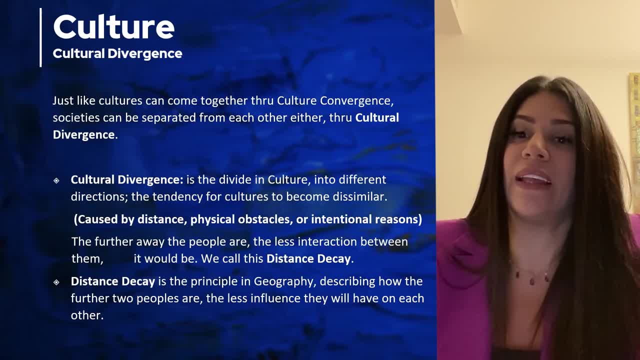 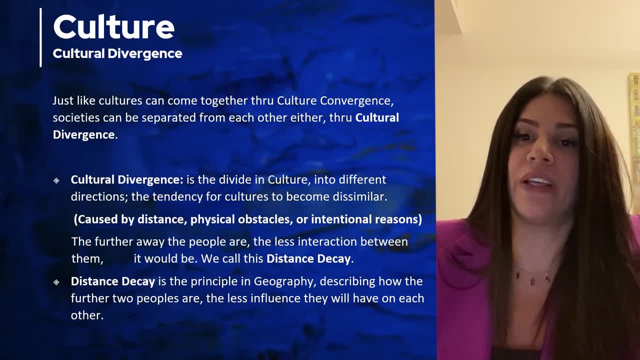 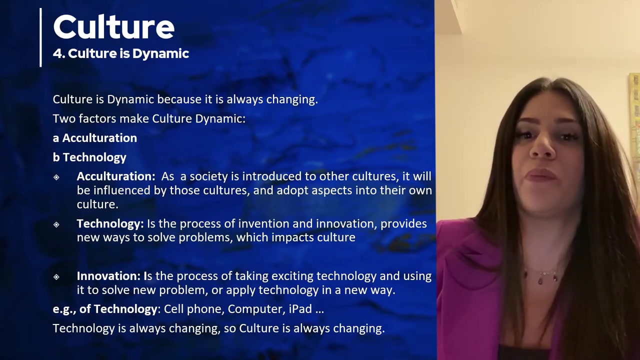 They don't accept modern technology as they worry about the influence of modern society. The separation between the Amish and the other communities is an example of intentional cultural divergence. Then we see that culture is dynamic. Culture is dynamic because it's always changing and all the time. 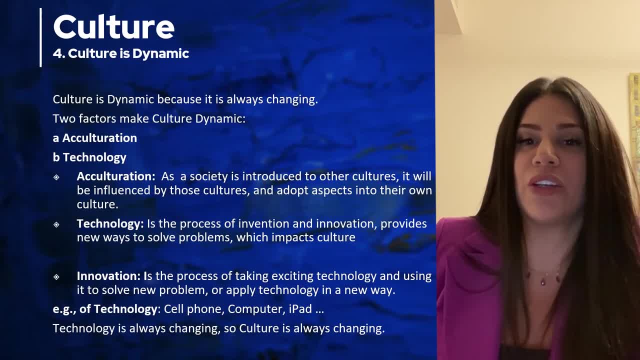 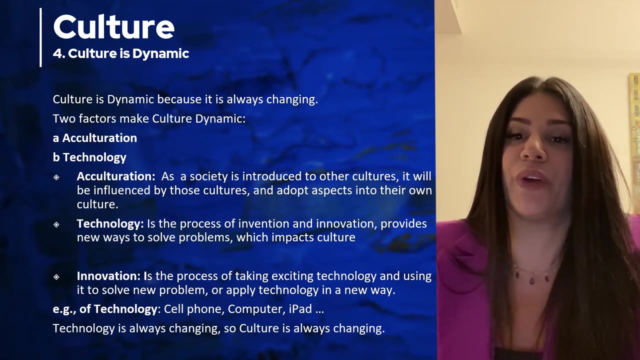 Why culture changes? Well, culture changes because of acculturation. As society is introduced to other cultures, it begins to adopt new aspects into their own culture. It might be food, music, language. So acculturation is the assimilation to a different culture. 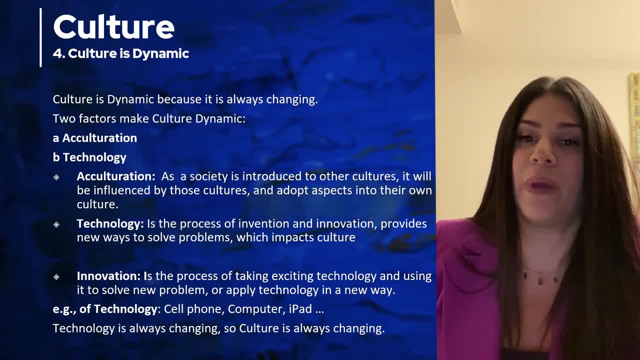 The other factor that makes culture dynamic and always changing is technology. So the technology is the use of scientific knowledge for practical applications in our everyday lives. Technology has strongly influenced the course of history and continues to do so. It's largely responsible for the change of our culture. 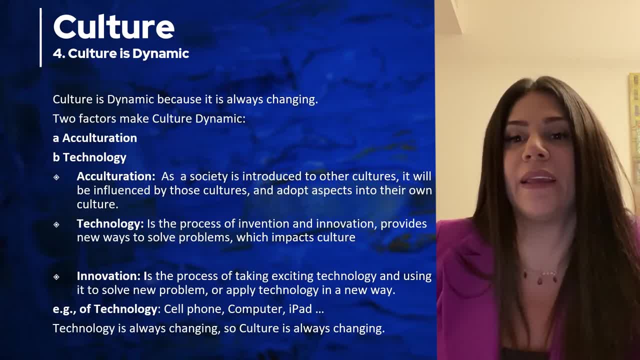 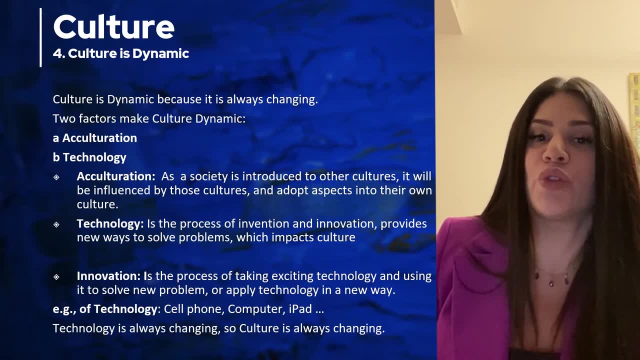 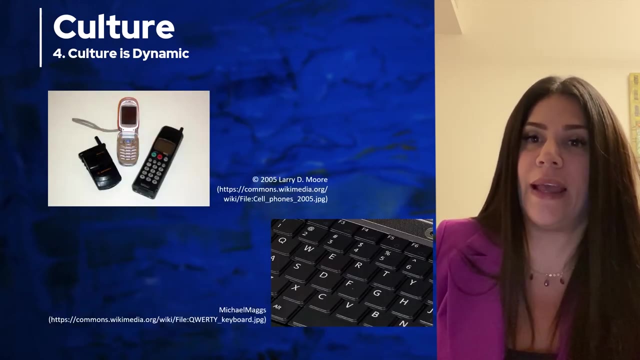 Now, innovation is the process of taking exciting technology, existing technology, and using it to solve new or apply it in a new way, Many times improving on that technology. Culture changes because of technology and innovation. To give an example, a great example of technology is the cell phone. 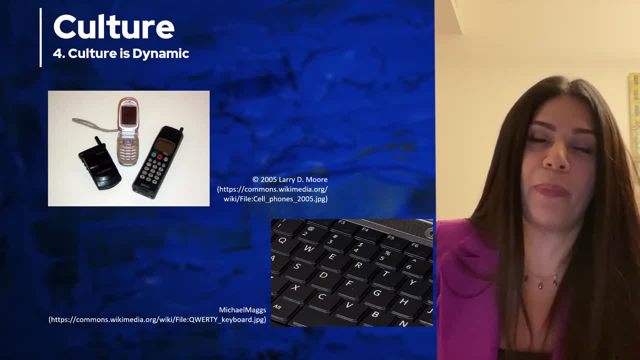 computer or iPad that I had when I lived in an apartment. I was working right in the city. When I lived in the city, the computer at the top and the Ipad the top of my TV. We wouldacionally shift technology. 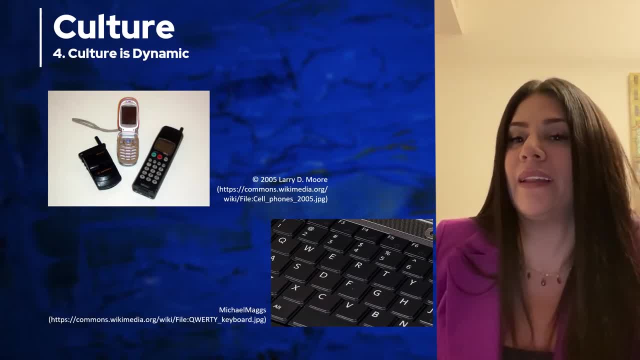 In high school I used to call my friends with the land phone with the extra long phone cord. Now we use the cell phone. Technology is always changing, so culture is always changing. We also find that culture is symbolic. Why culture is symbolic? 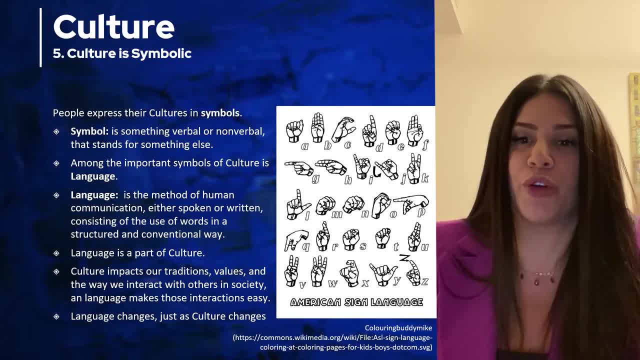 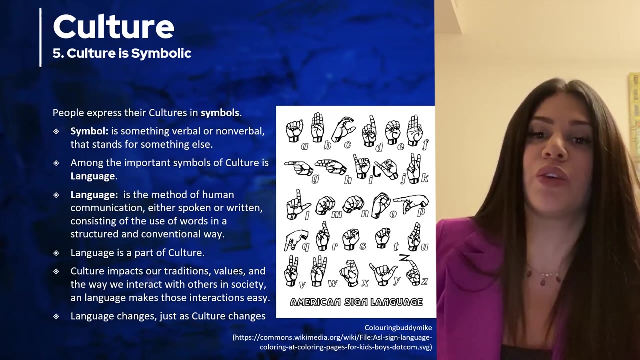 The symbolic is something verbal or non-verbal that stands for something else. Examples of culture symbols: the cross in Christianity, the star and crescent in Islam. People express their cultures in symbols. Among the important symbols of culture is language. So the language is the method of human communication, either spoken or written. 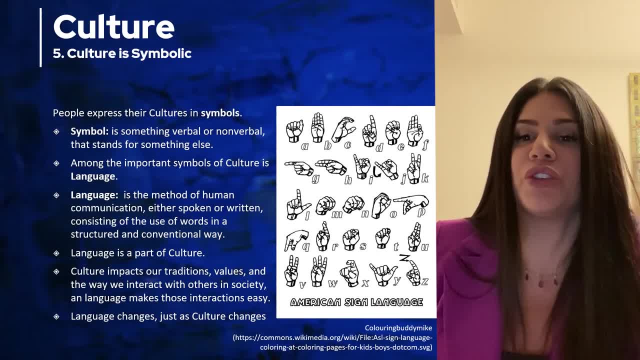 consisting of the use of words in structured and conventional ways. So there are over 6,500 languages spoken in the world. It's through language that we learn our culture, So language is a part of culture. Culture impacts our traditions, values and the way we interact with each other in society. 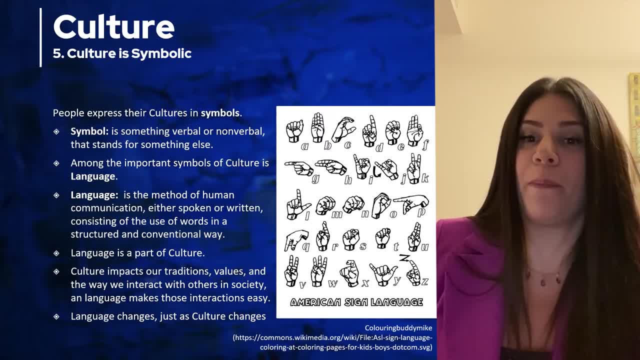 On the other hand, language makes those interactions easy. Language makes them защищ. escrito. Language keeps us active in common changes also, just as culture changes. for example, words are added to the english language or any other language every year. in 2018, the oxford english dictionary added more than 1100 new words. 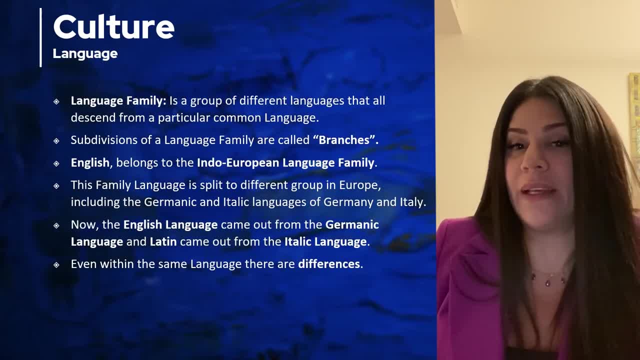 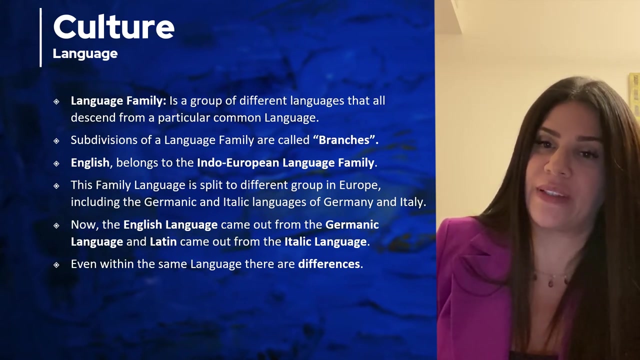 now we have a language family. a language family is a group of different languages that all descend for from a particular common language. subdivisions of a language family are called branches. english belongs to the indo-european language family, so language family is a language. so language family is a group of languages characterized by similarities and their evolution. 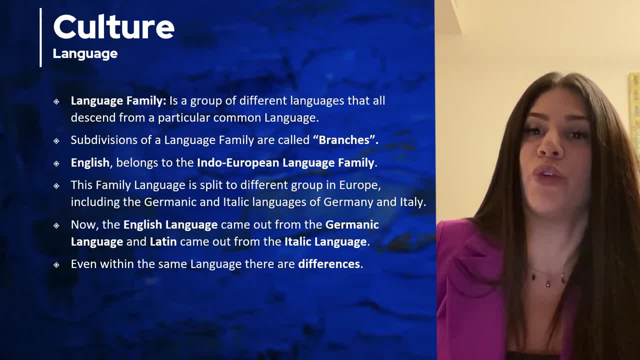 north european languages comes from the indo-european language family and because people they don't live at the same place in europe, this family language is split to different group in europe, including the germanic and italic languages of germany and italy. now the english language came out from the germanic. 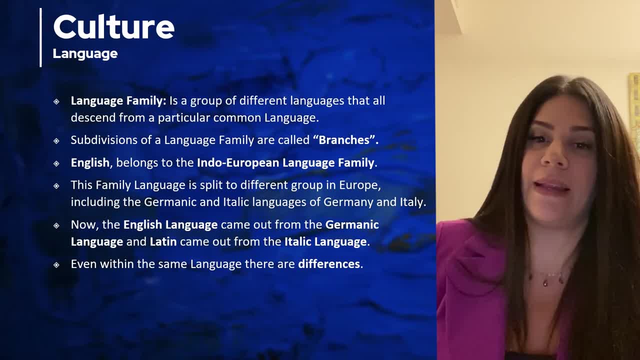 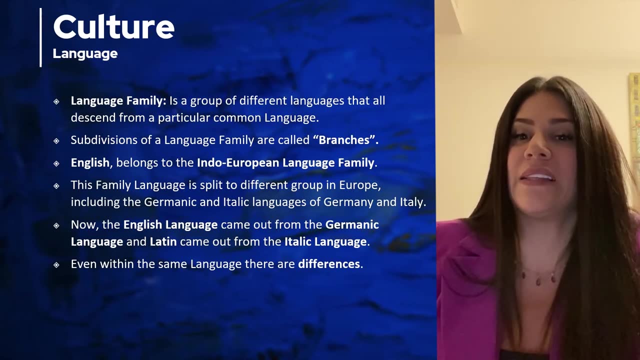 language and latin came out from the italic language. and even within the same language there are differences. if we will take the english language, between the american english and the united kingdom english. even we can still understand both languages. how we speak english in the united states is different than how we speak english in the united kingdom. 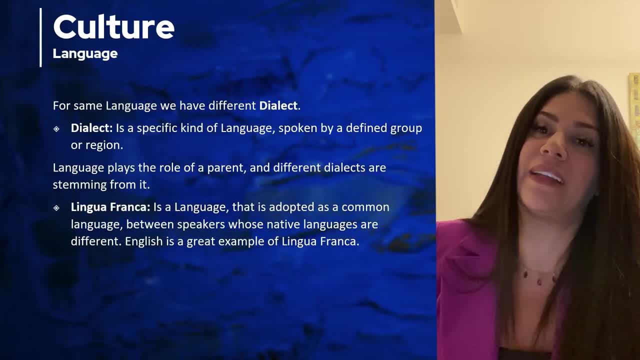 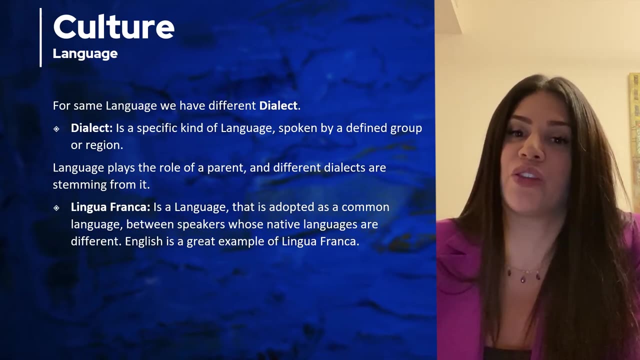 and for the same language we have different dialects. dialect is a specific kind of language spoken by a defined group or region. language plays the role of a parent and different dialects are stemming from it. so dialect changes in speech patterns related to class, region or other. 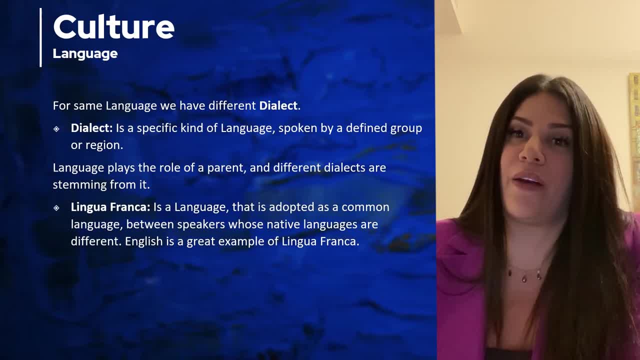 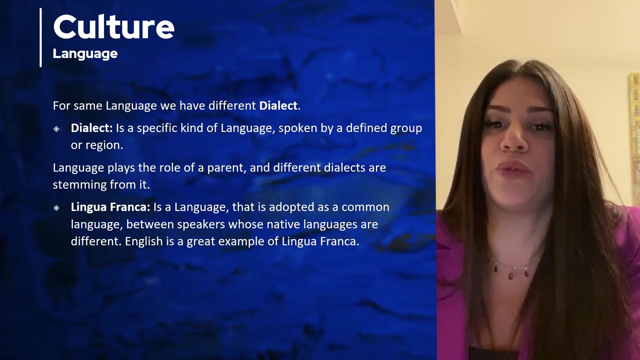 cultural changes and it's occurred in every language. now, with so many languages in the world and each language has its own dialects, works for 12 language like here, way or like that is the common language, or made of communication that enables people to understand one another regardless of their cultural and ethnical backgrounds. I'm Lebanese and I speak. 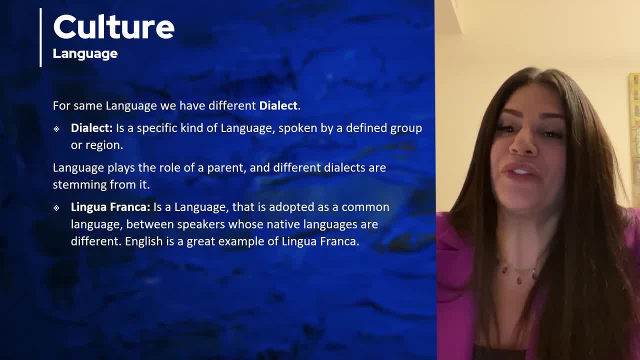 Arabic. in general, You are from different regions around the world and you speak different languages. The communication between us is English because English is a lingua franca language. Our communication is easy and understanding. Now let's move to the three different types of culture. 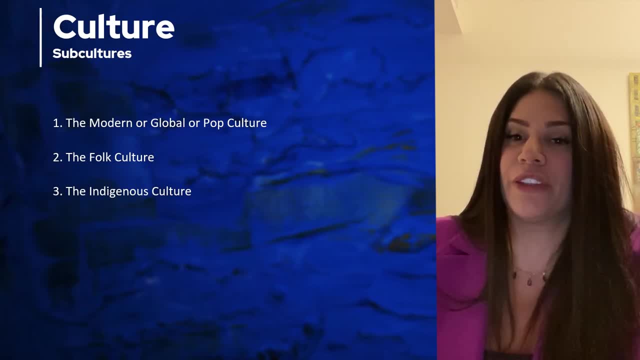 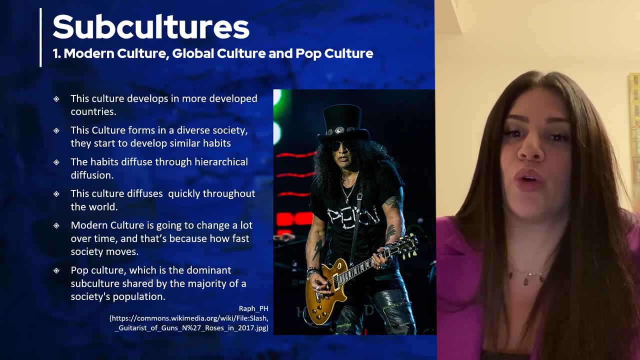 around the world. We have three different type of culture: The modern, or global, or pop culture, the folk culture and the indigenous culture. So the first one is the modern culture, or the global culture, or the pop culture. This culture develops in more developed countries. When we have wealth, we are able to see this. 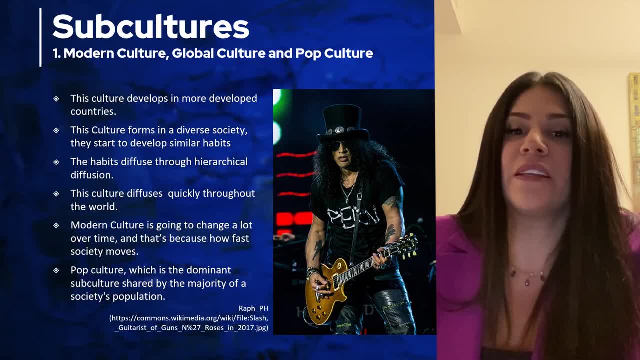 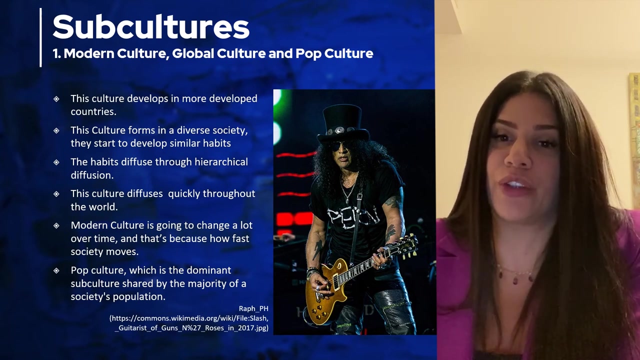 culture start to take off. This culture forms in a diverse society. They start to develop similar habits and these habits diffuse through hierarchical diffusion, The internet. this culture diffuses quickly through the world and diffuses through areas that have access to wealth. Modern culture is going to change a lot over time and that's because how fast society moves. 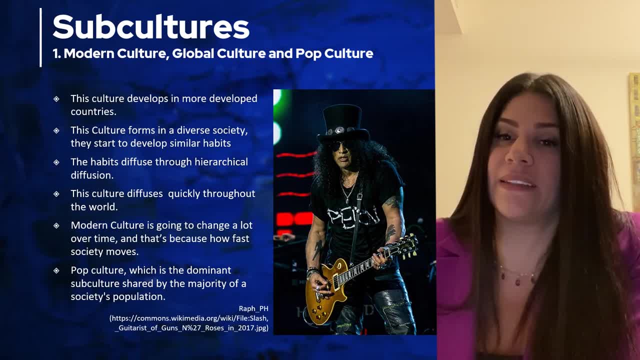 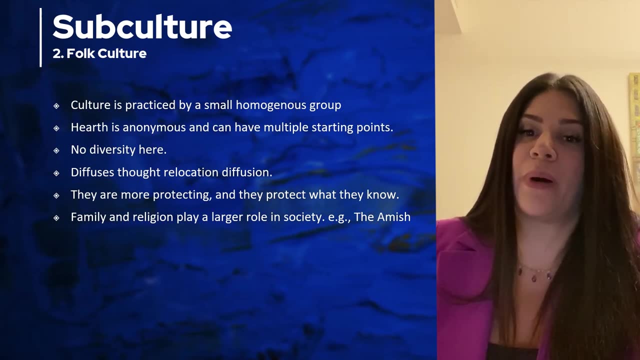 That's why some people are hesitant or try to prevent modern culture from influencing other people- their own. the second type is full culture. full culture is practiced by a small, homogeneous group. we don't have a lot of diversity here. this culture diffuses through relocation, diffusion. there are, they are more protecting and 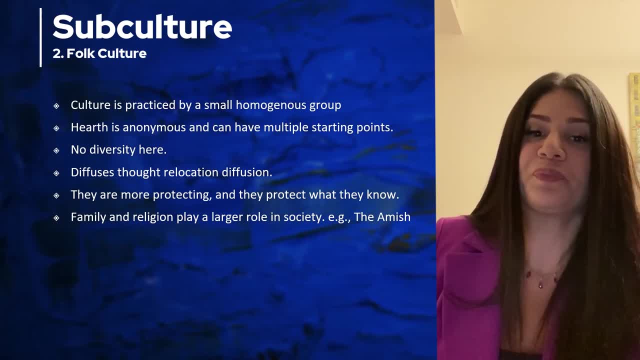 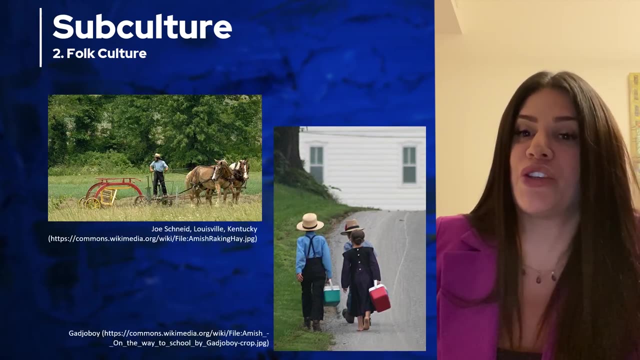 they protect what they have, what they know, where family and religion play a larger role in society, the Amish, for example, are a great example of a full culture. the Amish came from Switzerland, Germany and France. they migrated to the United States. they just trying to protect what they have. they don't care. 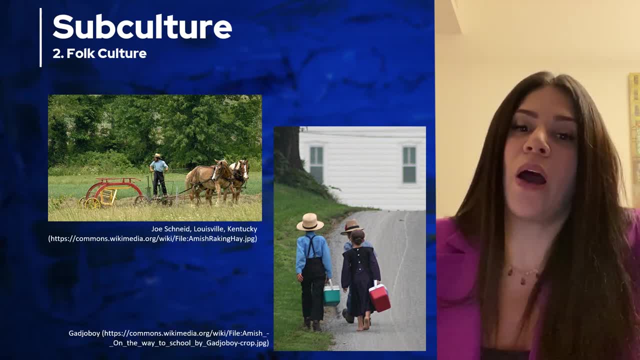 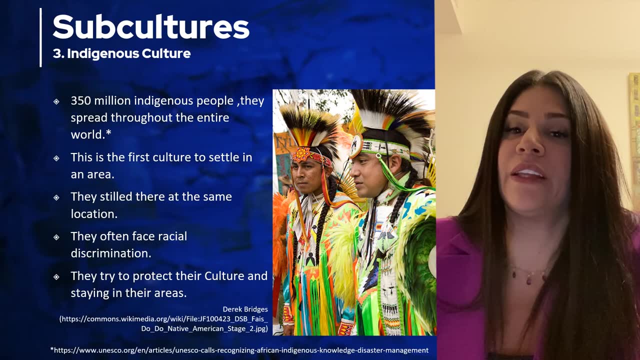 about gaining numbers. our third culture is the indigenous culture. there is 350 million indigenous people in the world and the third culture is the indigenous people in the world. they spread throughout the entire world. when dignity was, culture is referring to the first people that settled in an area, so 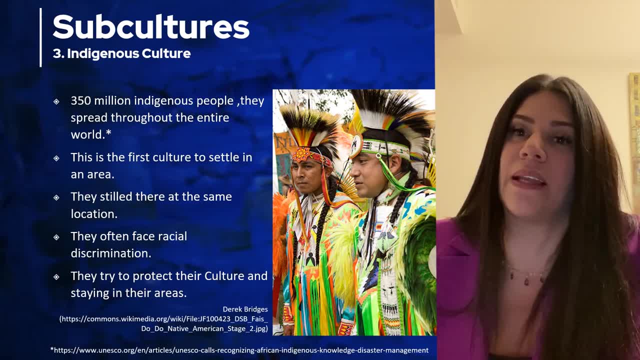 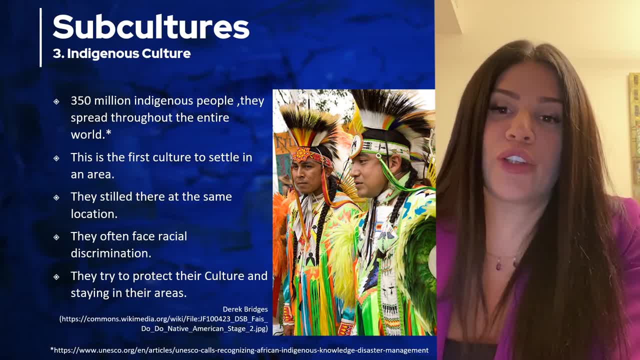 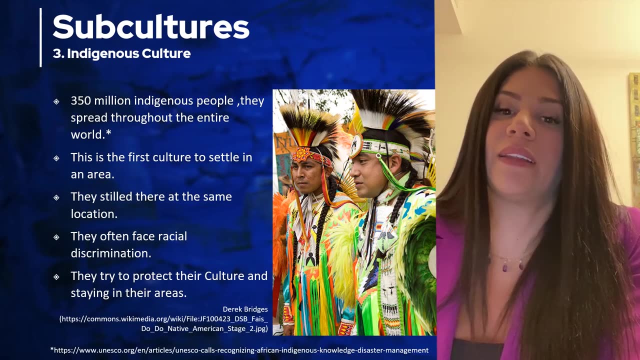 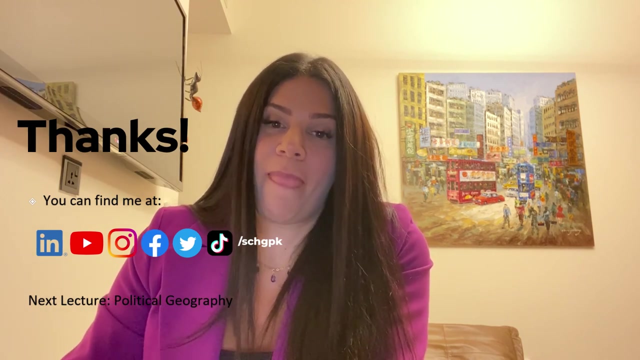 discrimination. they are going to protect their culture as best they can. they are trying to stay in their areas. they are not going to be changing as much over time unless there are outside forces that are impacted them. so those are the three different classification of culture. so now you should understand that culture is we talk about. what is culture? the components.